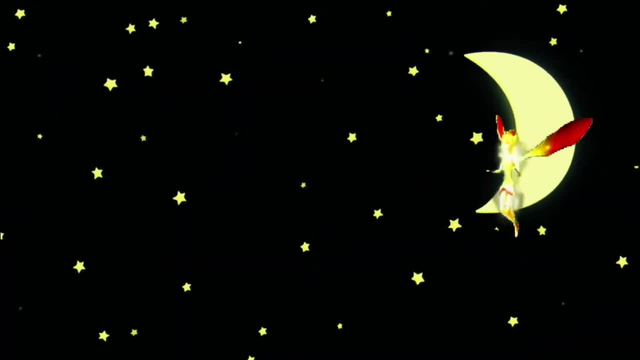 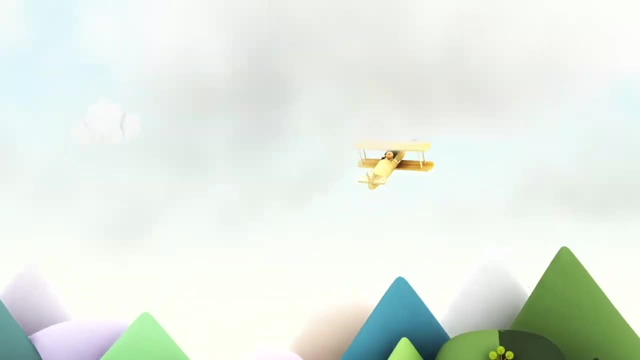 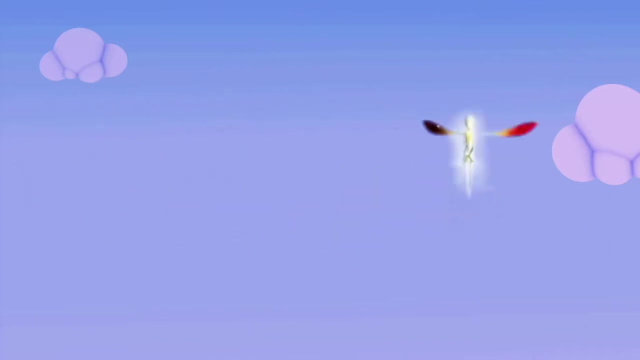 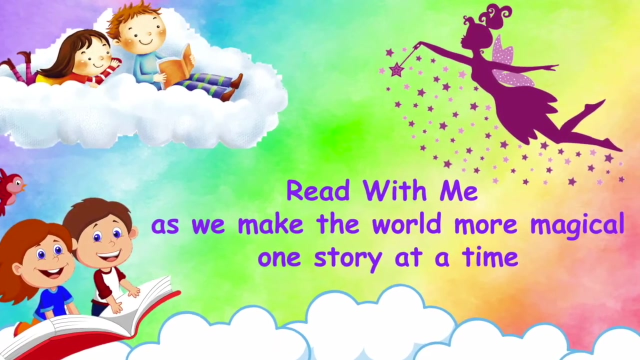 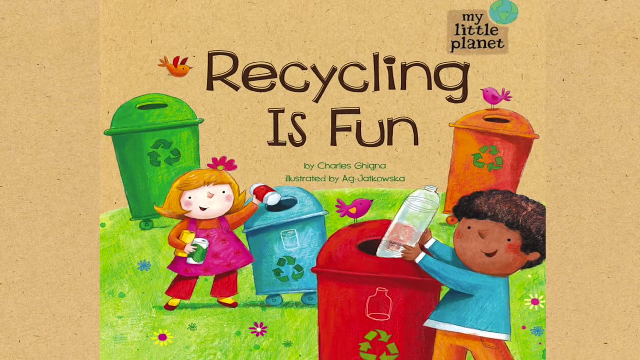 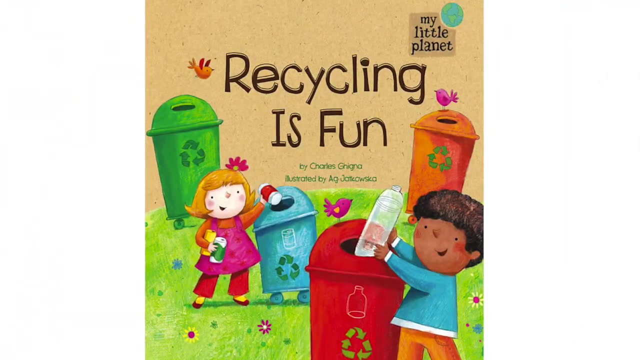 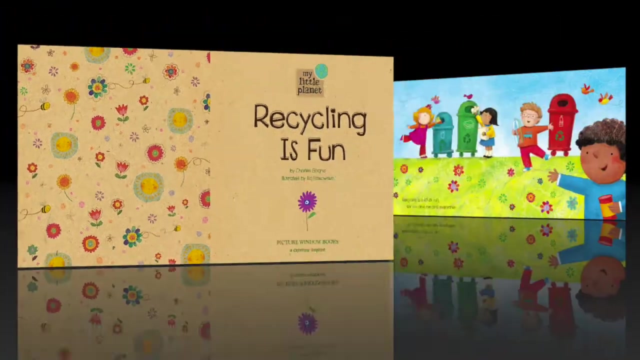 Hey there, Are you ready for today's story? Let's go My Bedtime Stories. Read with me as we make the world more magical, one story at a time. Recycling is fun By Charles Gignac, Illustrated by Agjet Koska. Recycling is a lot of fun for you and me and everyone. 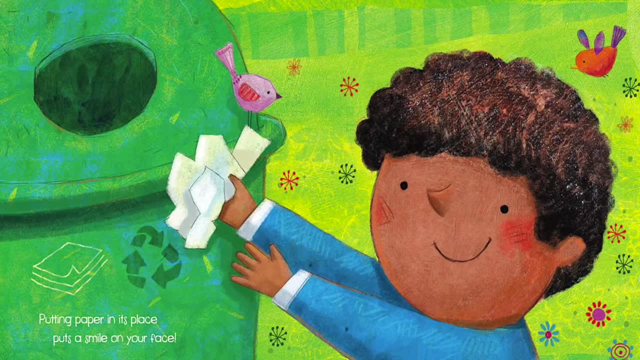 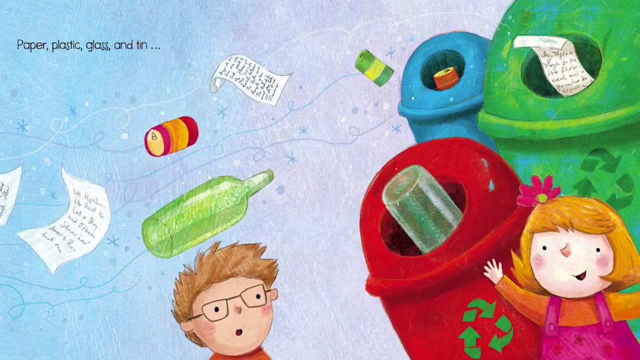 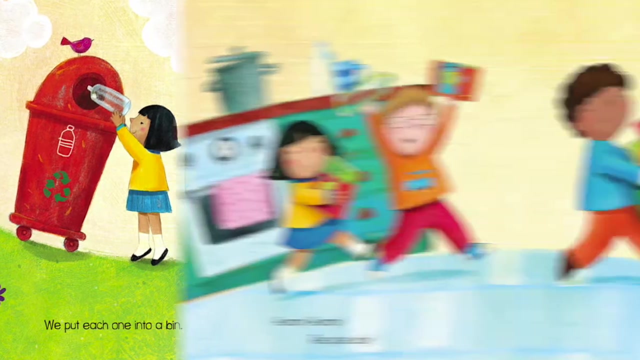 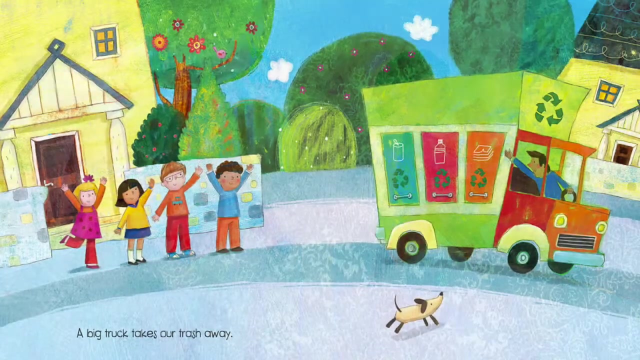 Put it in the comment section below: Putting paper in its place puts a smile on your face. Paper, plastic, glass and tin: We put each one into a bin. Hooray, Hooray, Recycle day. A big truck takes our trash away. 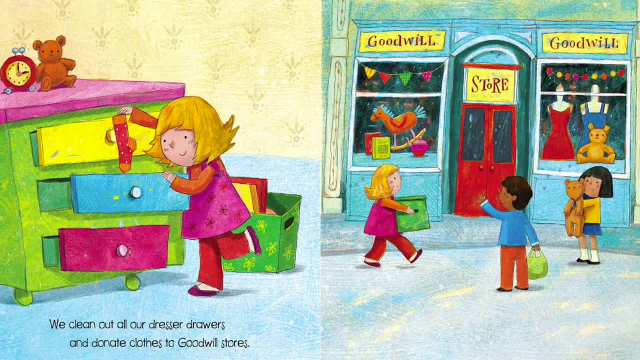 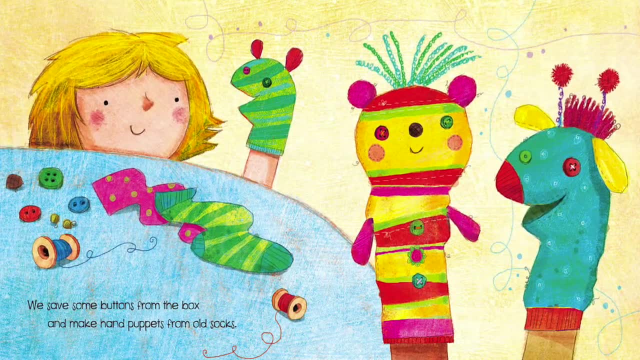 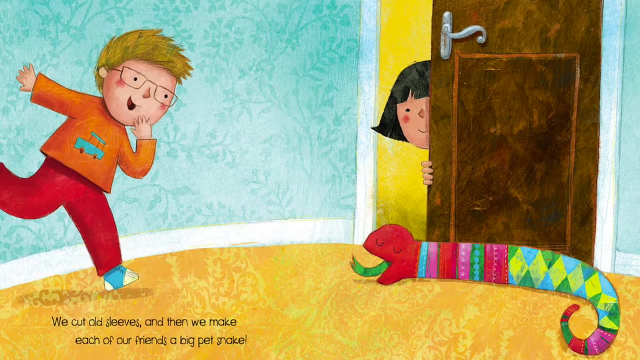 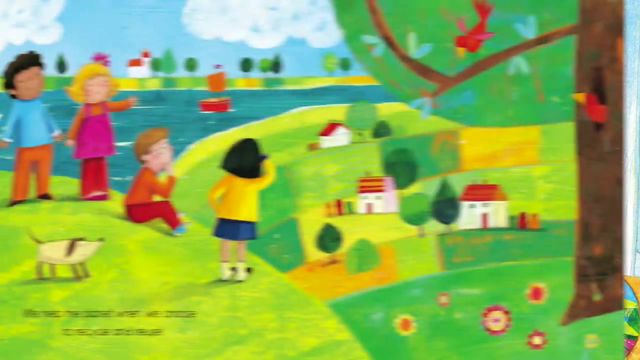 We clean out all our dresser drawers and donate clothes to Goodwill stores. We save some buttons from the box and make hand puppets from old socks. We cut old sleeves and then we make each of our friends a big pet snake. We help the planet when we choose to recycle and reuse. 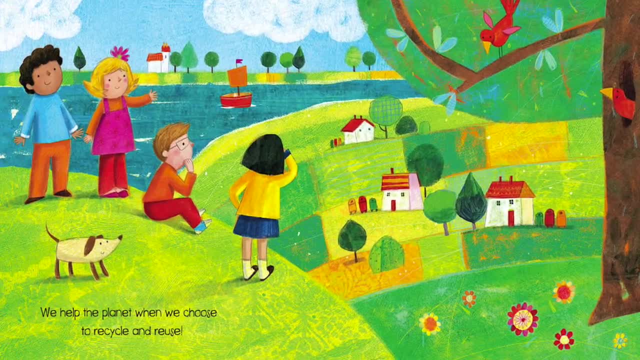 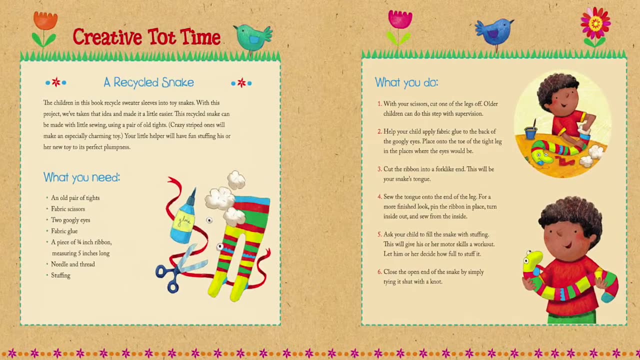 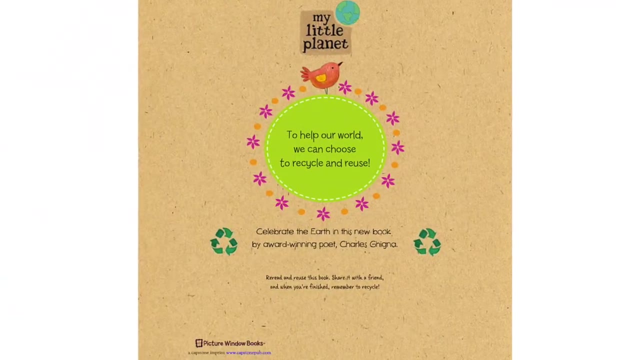 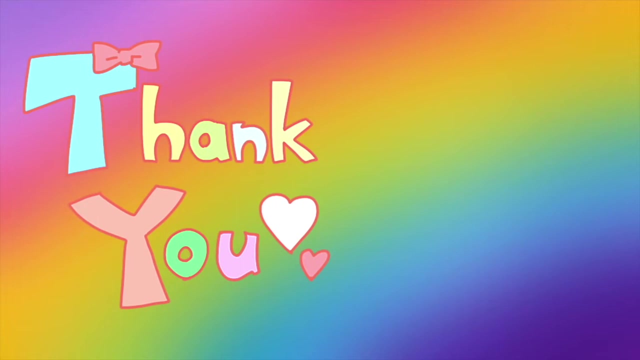 We help the planet when we choose to recycle and reuse. We care for nature when we do the laundry, like Sarah the banana. Our plans are waiting for you. Thank you so much for staying and reading with me until the end. Please give this a thumbs up if you enjoyed this and share it with your friends. 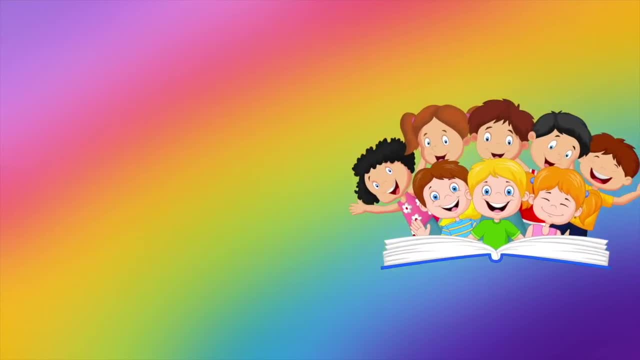 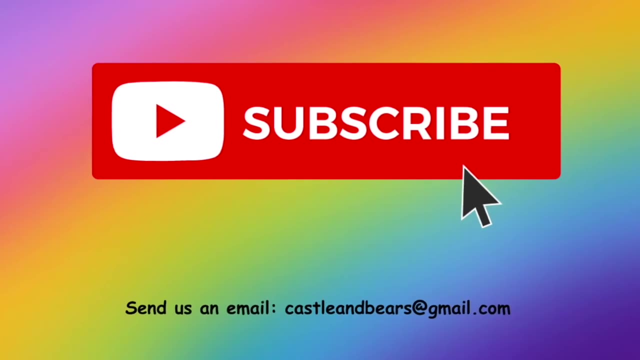 so we can all read along together. All performances want to add to your savings and help your plans along together. See you on our next one. Bye.